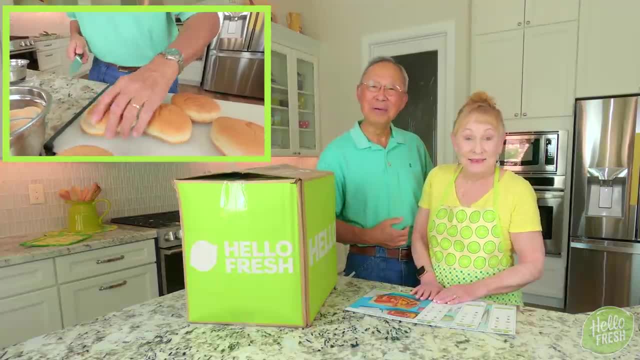 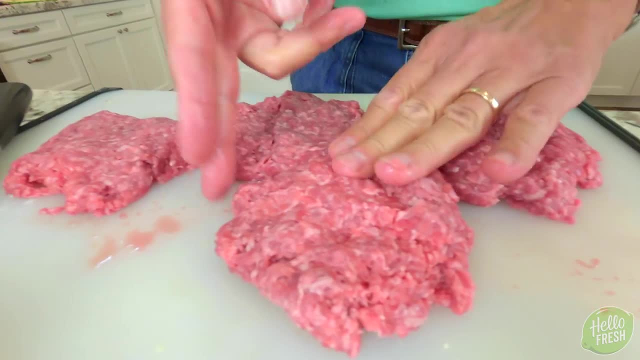 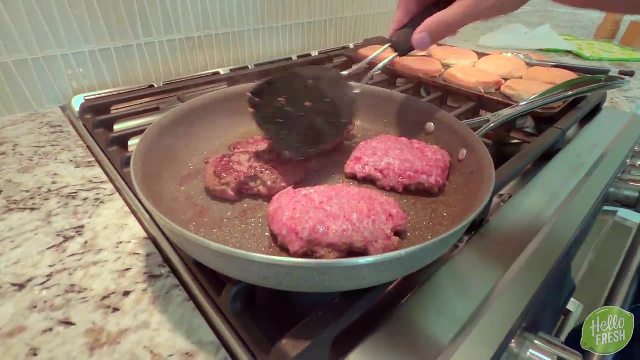 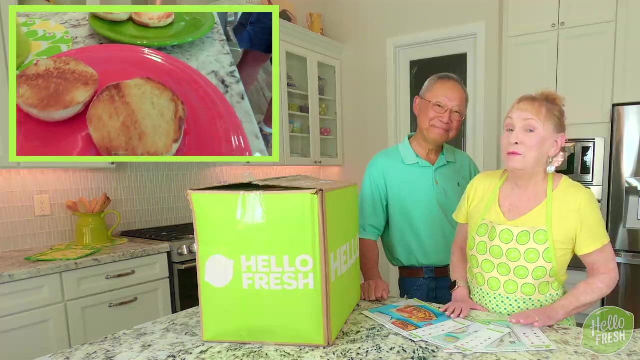 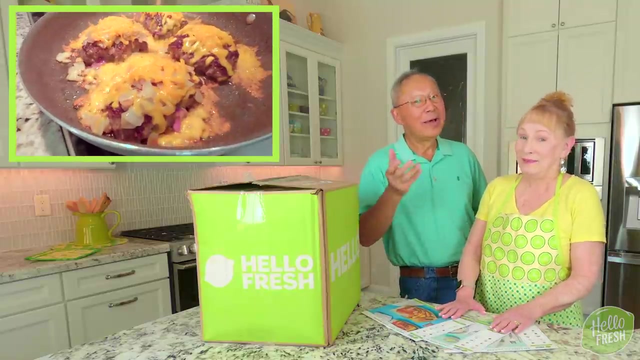 The recipes are so delicious and it saves time and it has become part of our routine. I'm a very picky eater, but the Hello Fresh food is so delicious And I'm a big eater, so Hello Fresh allows me to choose a bigger box size. 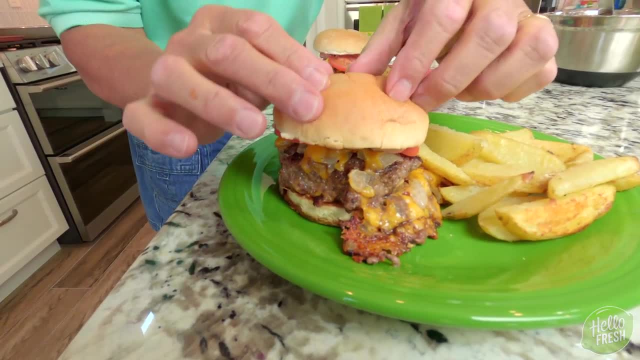 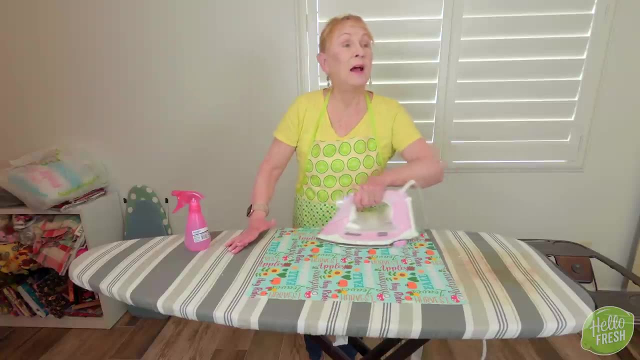 The best way to spend time in carbonara is with a plate. If you don't have a plate, you can make a bag, or you can just put it in a electric grill. The most delicious food is cooked in the oven. It's so good it makes me hungry. 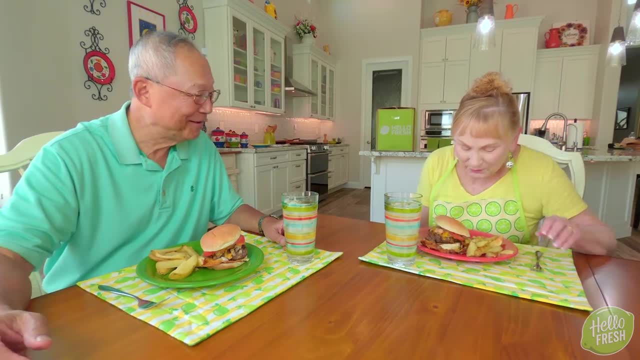 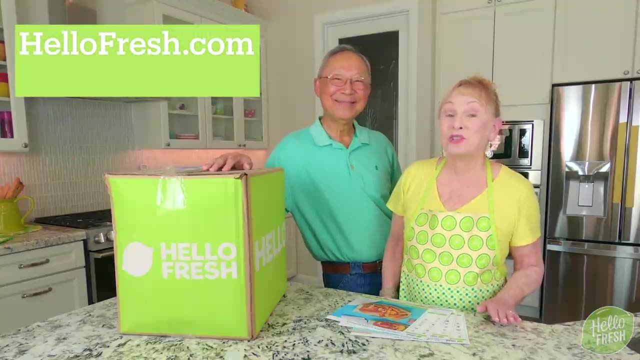 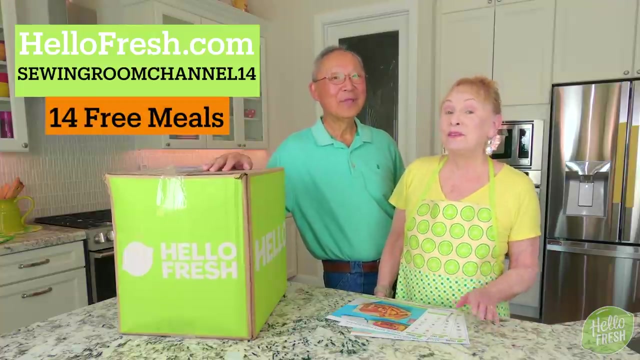 Cheryl dinner's ready. Okay, I'll be right there, Boy, this turned out great. It smells so good and I'm starving To try Hello Fresh. go to hellofreshcom and use code SewingRoomChannel14 to get 14. 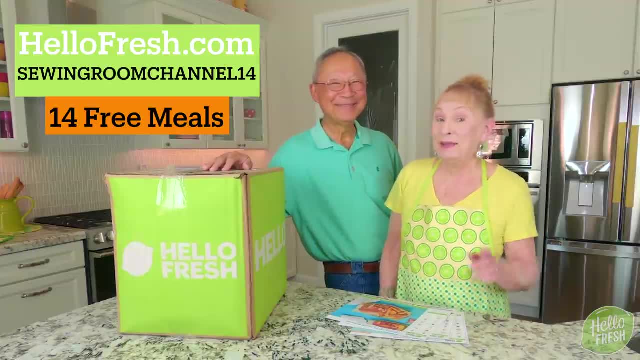 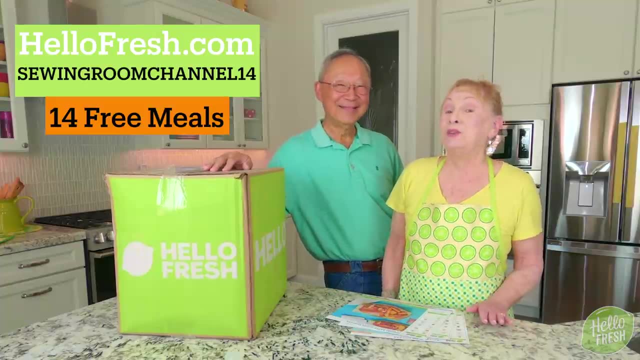 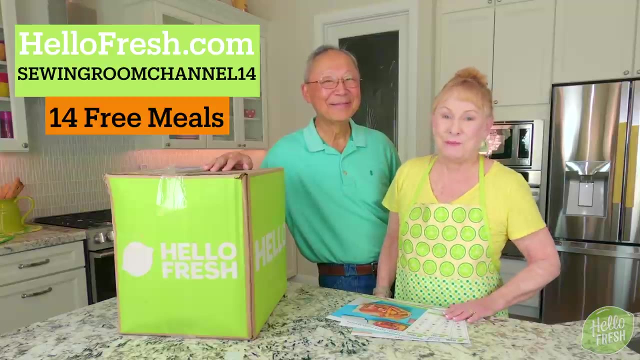 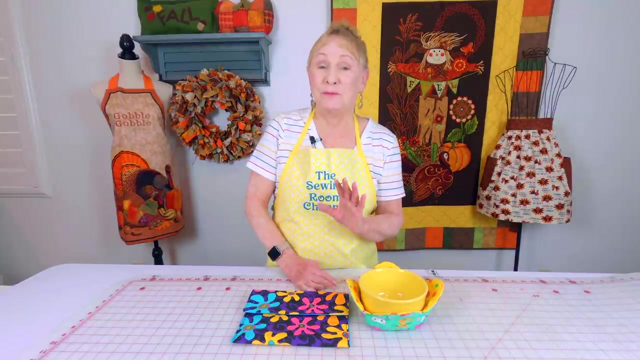 free meals and free shipping. Now make sure you write that down. To try HelloFresh, go to HelloFreshcom and use code Sewing Room Channel 14 to get 14 free meals and free shipping. That food was really, really good. Now, speaking of cooking in the kitchen, I have two items. I'm 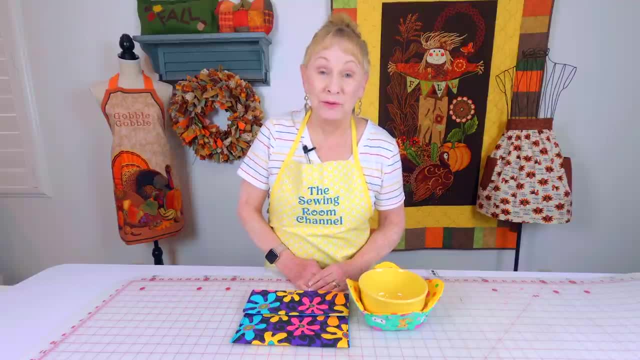 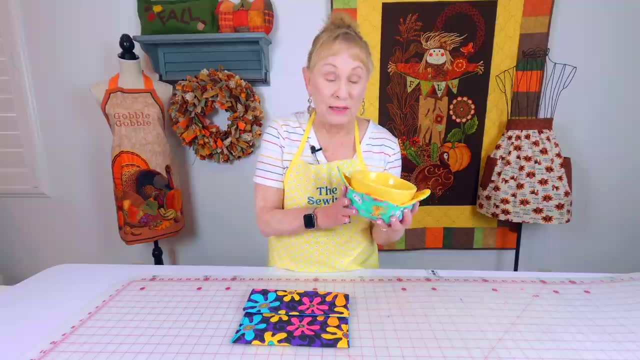 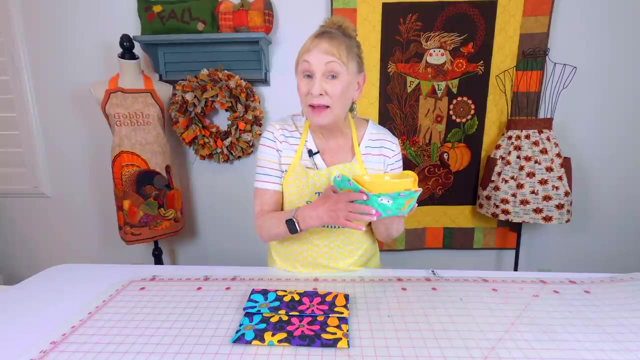 going to show you how to make. that will make your cooking process in your kitchen so much easier. And this is a microwave bowl cozy, So when the bowls are super hot, you pull them out of your microwave and you won't burn your little fingers. And they are pretty too. And this other one, I 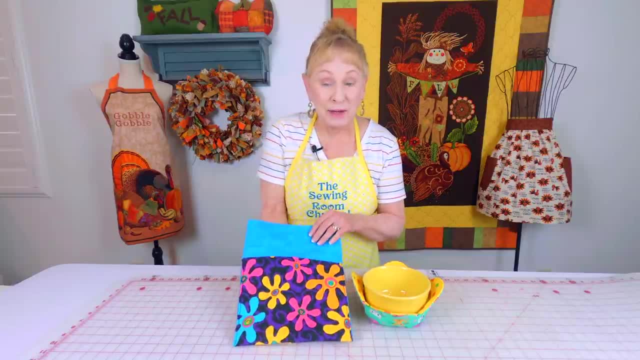 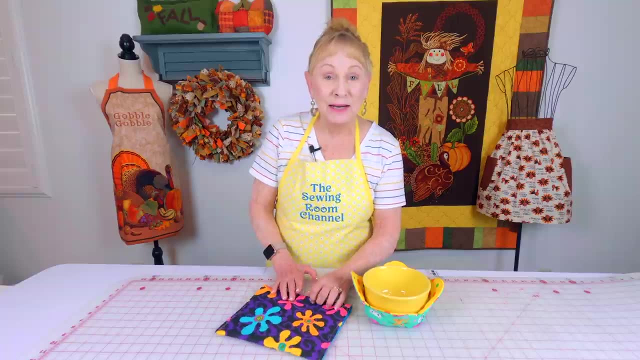 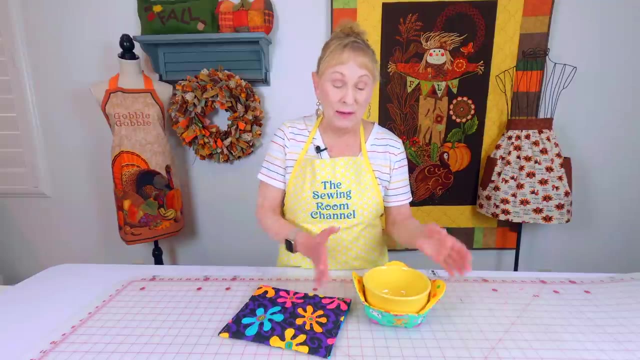 really, really love, And it's a microwave potato cooking bag. You just slip your potatoes in there, close it up, Turn it upside down and cook. Now I am using fat quarters. I use two different ones for this one and two different ones for this one, But you can use all the same fabric if you like. 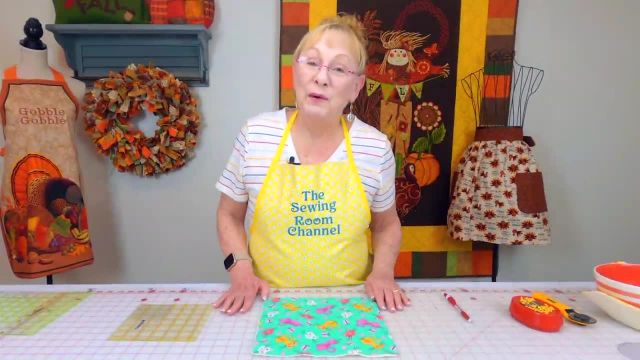 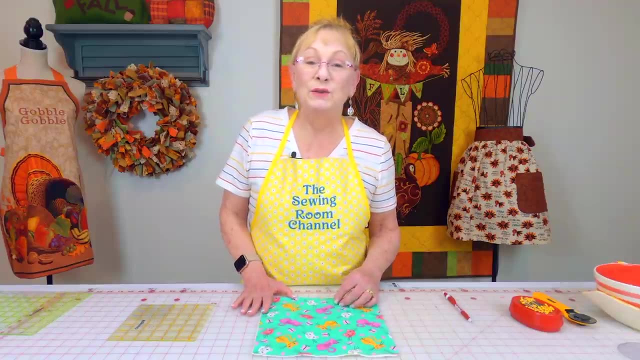 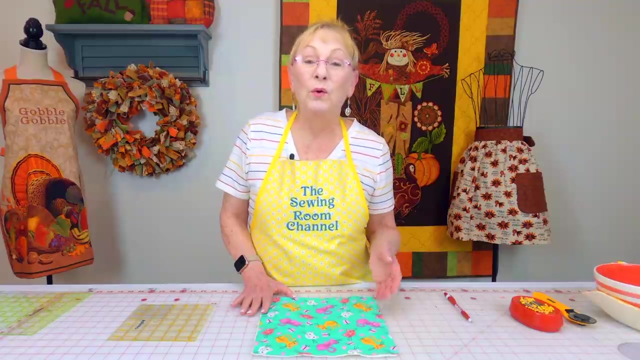 So let's get started. For the microwave bowl cozy, I'm using quilting fabric that's 100% cotton, So you're going to need two squares that are a 10 inch square. It can be the same color or a different color. Then you're also going to need two squares that. 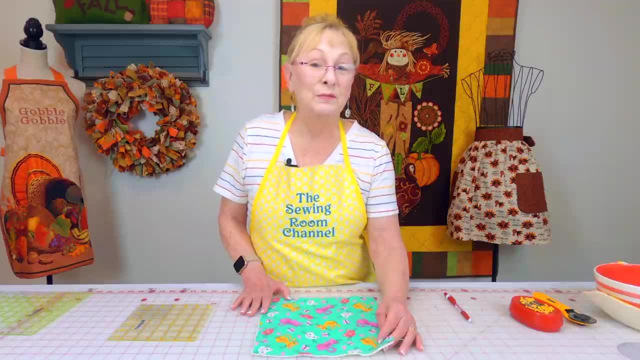 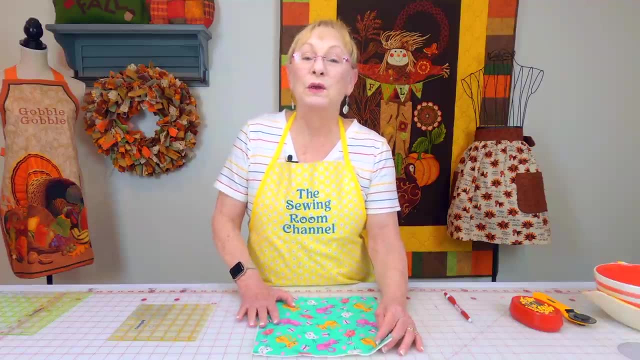 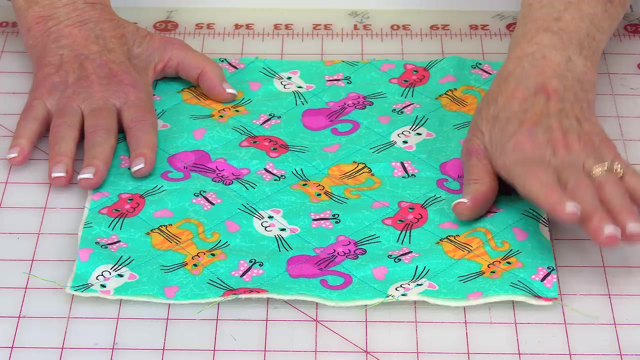 are 10 inches by 100% cotton batting. Don't use anything polyester in this, because it is going into your microwave. Also, use 100% cotton thread. So you're going to take one piece of cotton batting and lay it down, and take one of your squares and place it on top with the pretty. 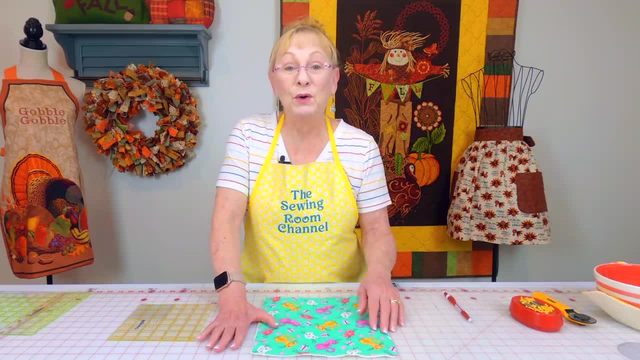 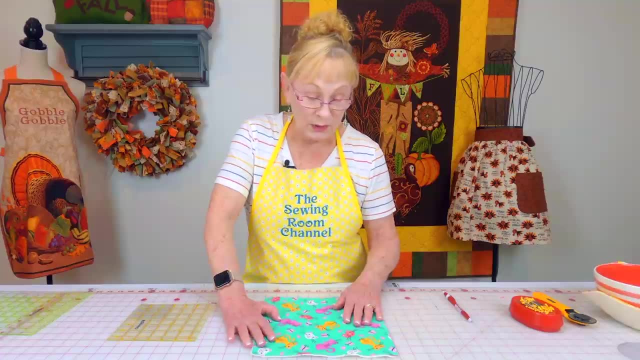 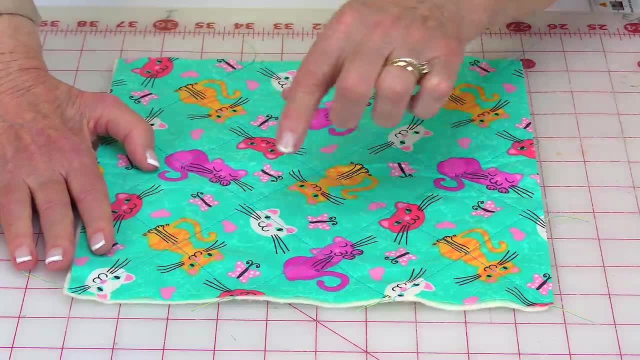 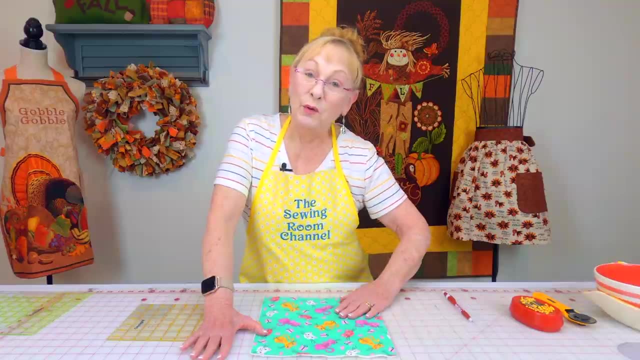 from corner to corner. and then I went out and did another stitch- a couple of inches- and then went out and did one more, a couple of inches. Then I went over and did the same thing on the other side. Then I turned it and did the same thing on the other side. 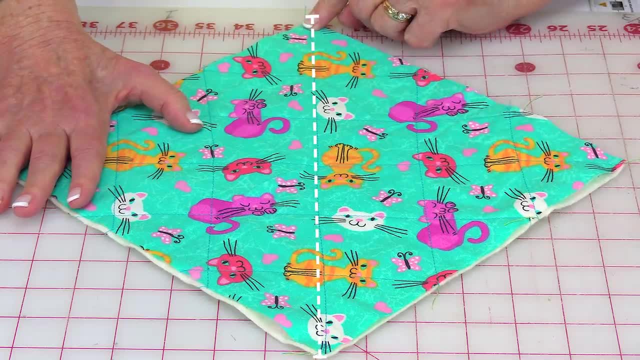 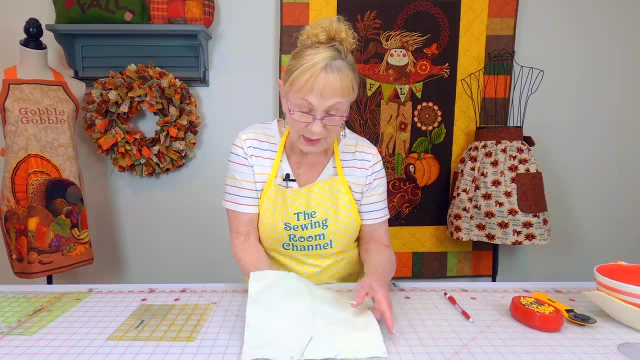 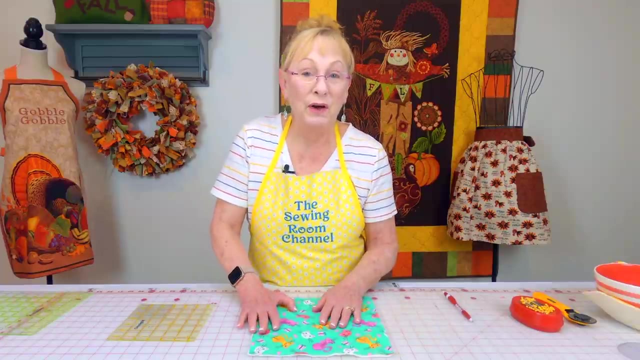 Going down the middle first and then going out and doing two more rows. So it's on a diagonal pattern. I'm going to show it to you on the back. You could probably see the stitches a little better. You do that with both of your cotton battings and both of your cotton squares of. 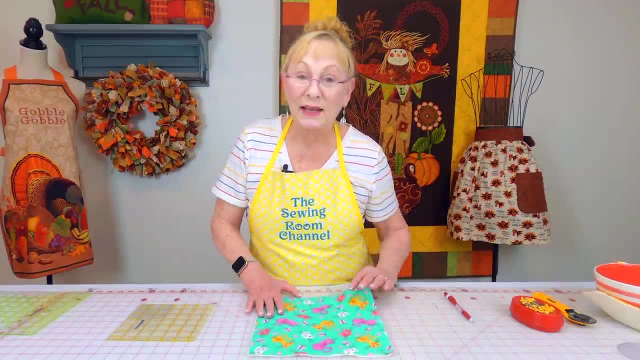 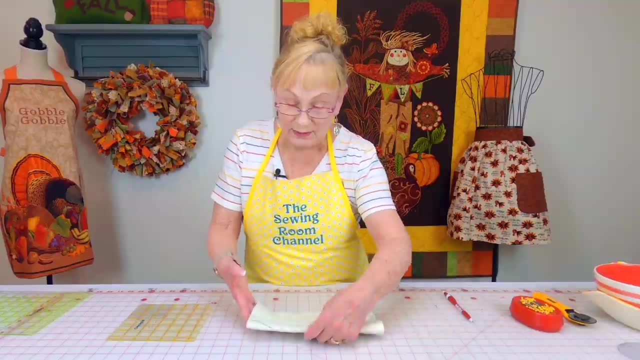 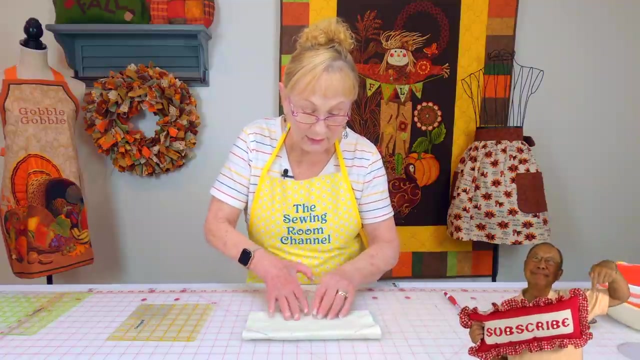 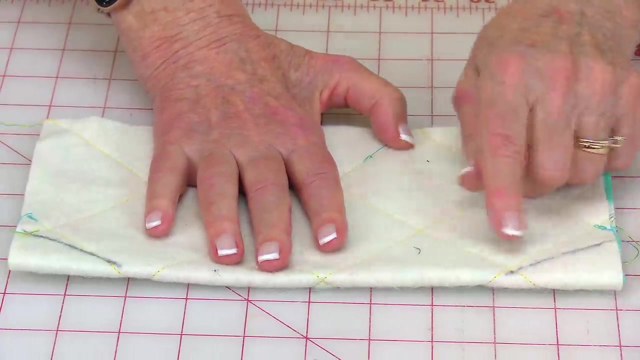 quilting fabric. Then you're going to take it and fold them in half And I'm going to show you how to put some lines on it. Now, down here at the folded edge, make sure it's lined up here at the top. So down at the folded edge, make sure your fabric is smooth on the inside. You're going to 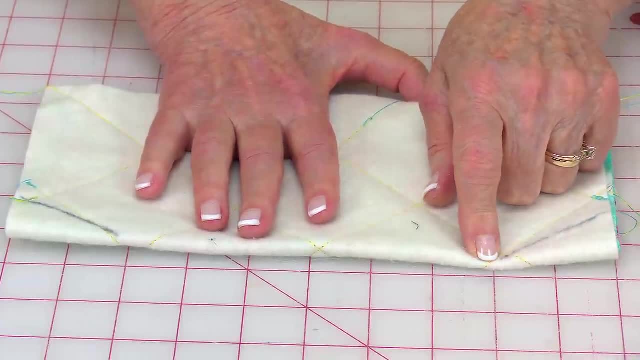 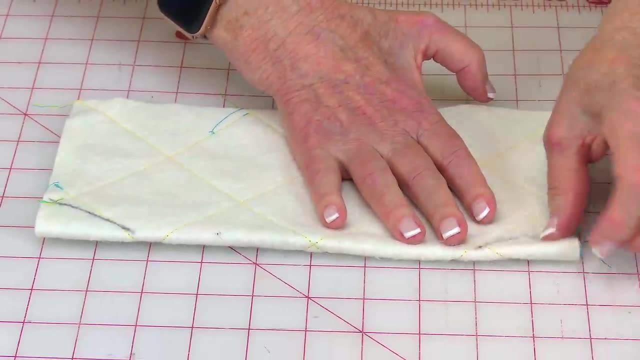 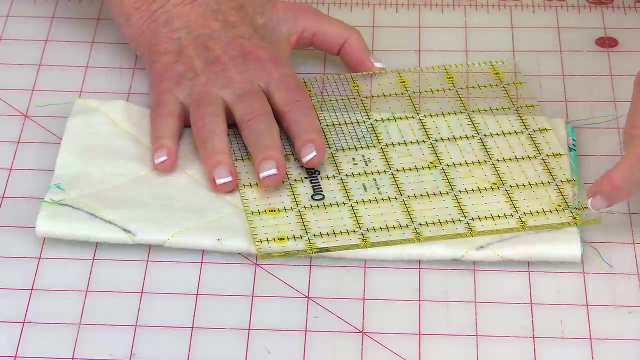 go over two inches this way and then up one inch this way, And I like to use the lines on my cutting mat, So I've pushed it into the corner here And I'm taking a little bit of the fabric and I'm taking a ruler and putting it down here up against the one inch going up this way And then over on. 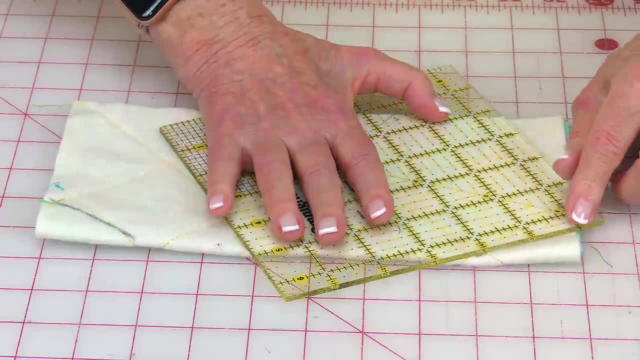 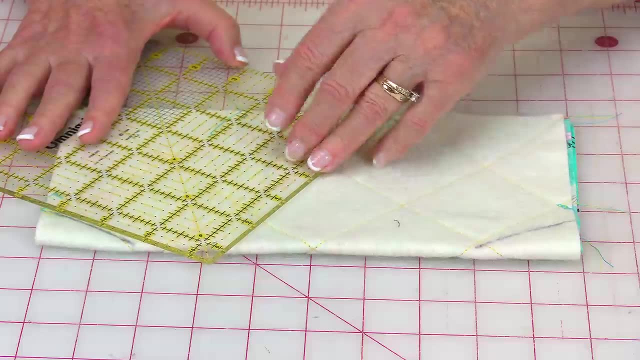 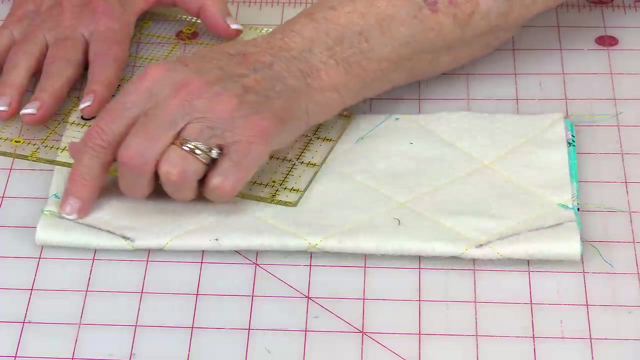 the two inch going that way. So one and two, Just remember that. And then draw a line, Go over here to the other corner and do the same thing. Then you're going to stitch right on top of that drawn line, on both edges. You're going to trim some of this off, So I'm going to do a little bit of a. 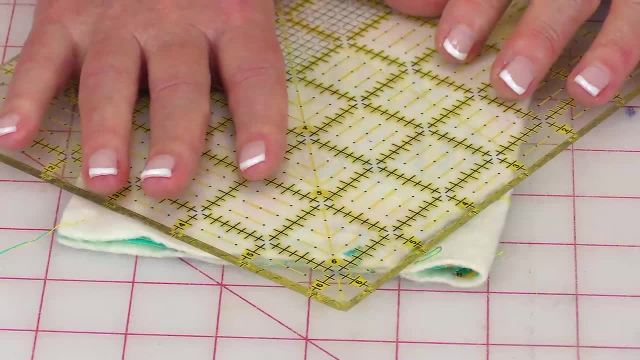 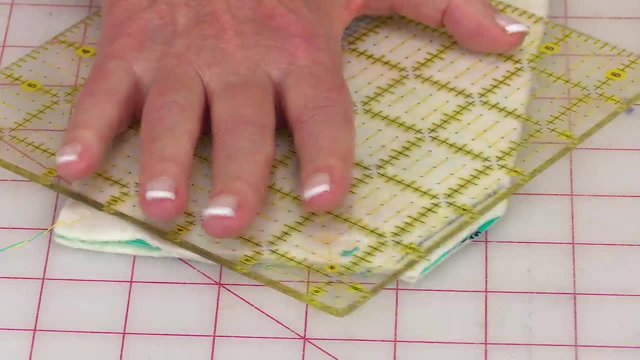 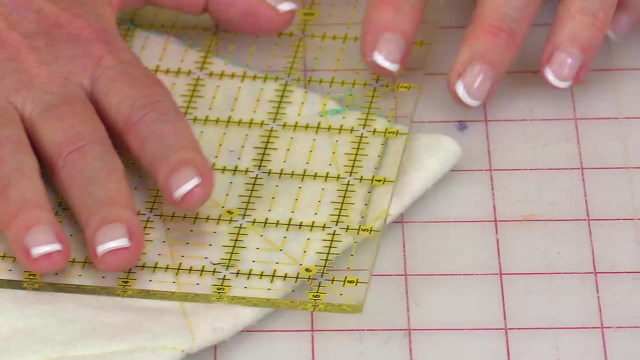 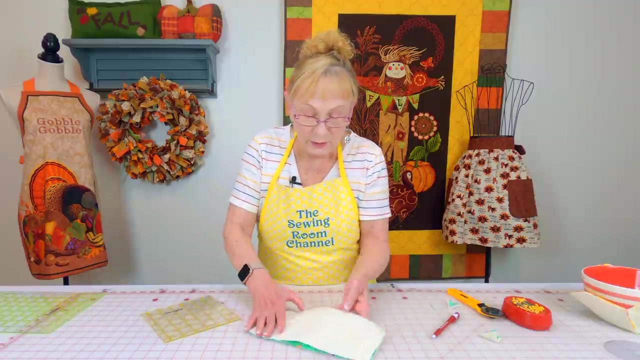 turn. I'm placing the quarter inch line on my ruler right on top of that stitch line And I'm going to just trim it off with my rotary cutter. Then I'm going to turn it and do the same thing on this corner And cut it off. Now take your bowl cover and open it up, And now you're going to turn it. 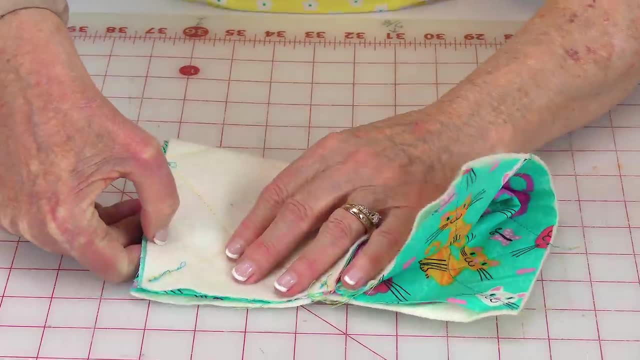 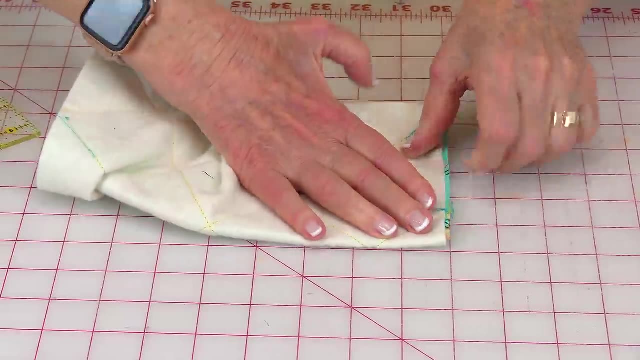 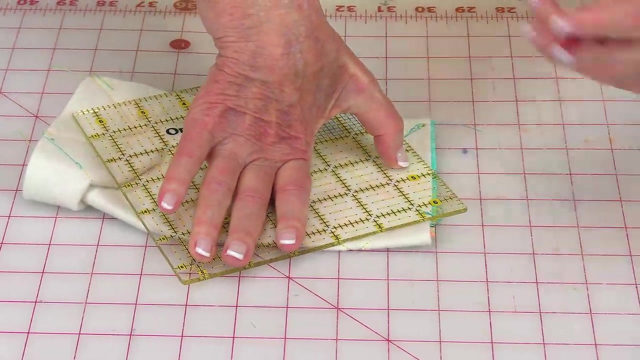 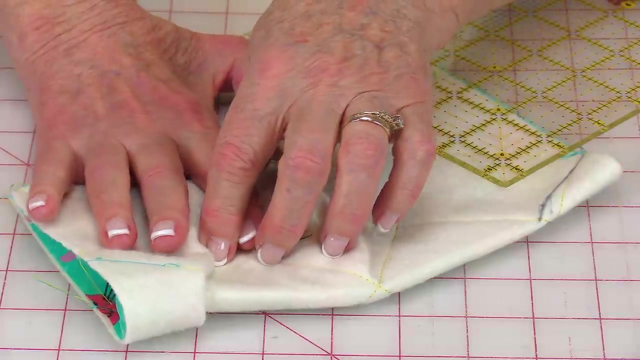 and fold it this way And you're going to repeat the same steps. You're going to draw those lines from the one inch to the two inch And then go over to this corner and do the same thing, Then stitch on top of those lines and then trim the excess off. 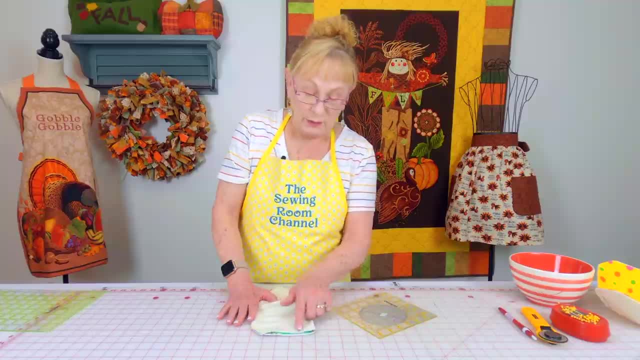 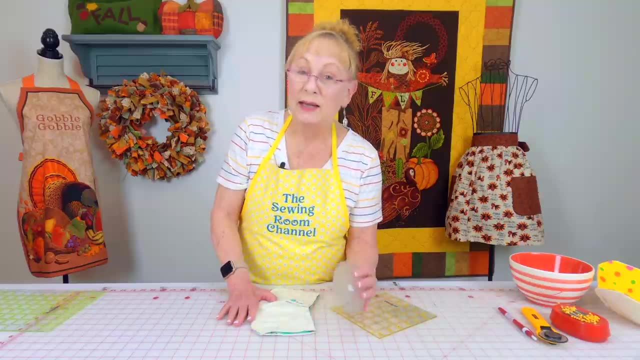 You have two ways you can do this. You can leave the corners pointed like this, Or you can round them. So I like rounding them. So take anything round A large lid, whatever you have handy, And when the side of your lid or 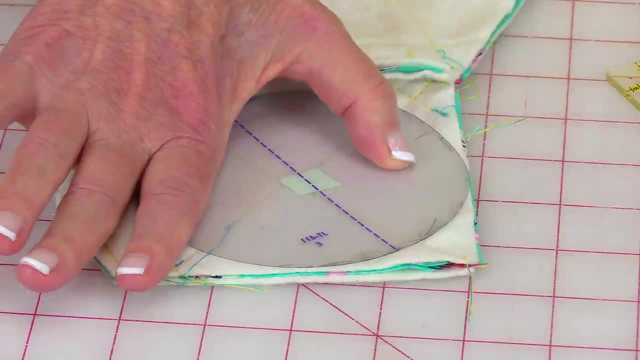 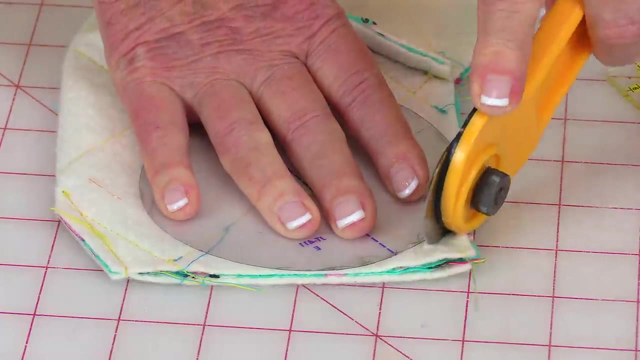 whatever template you're using touches the edges, then either draw around it and then cut it with scissors. I'm just going to use my rotary cutter And I'm just going to trim right around it like that And then go over here to this side and do the same thing. 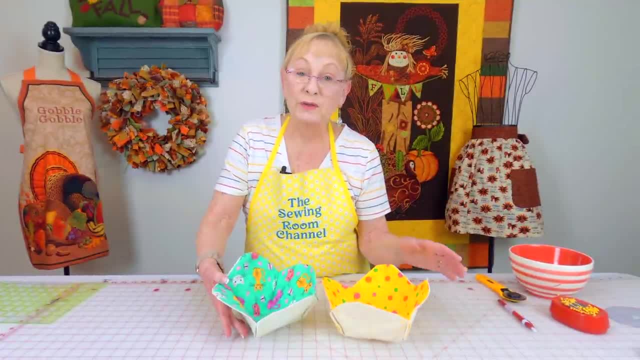 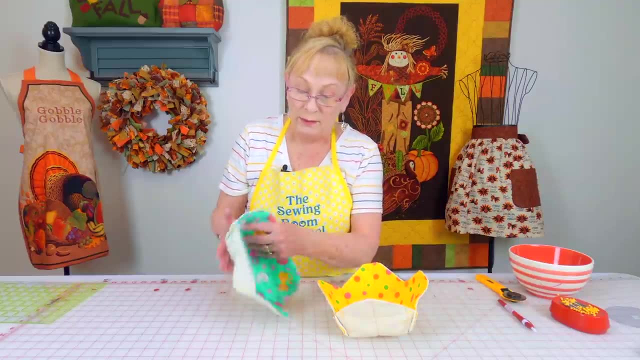 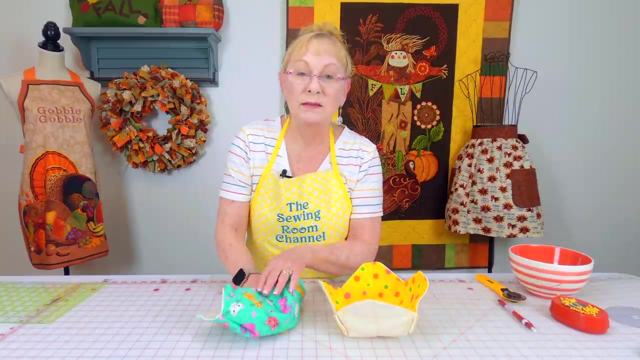 So you're doing it to both of your squares and cotton batting, So you should have two of these when you're done. You want to turn one to where one is outside and one is inside. So this: on this one, the outside fabric is showing. On this: 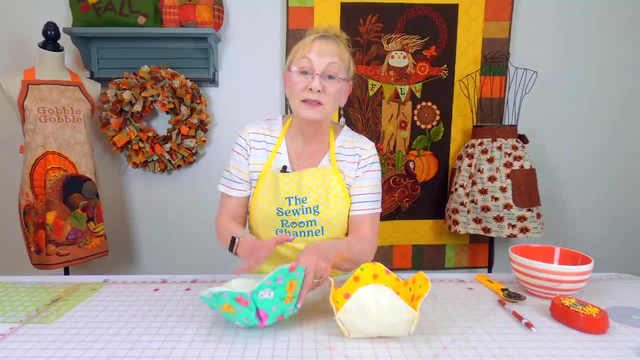 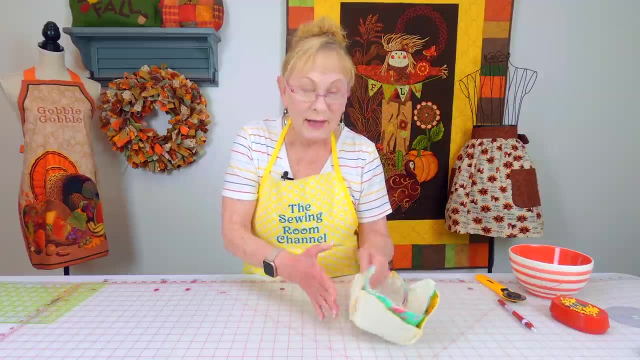 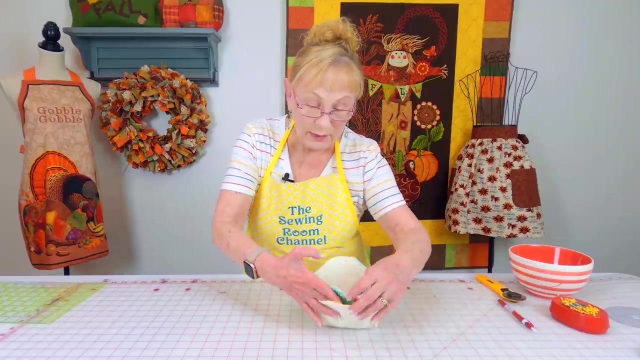 one the cotton batting is showing. We're doing that because we're going to stitch them together, So you want to take them inside of each other. so when you're looking at it now, you're seeing both cotton batting sides. Then you're going to line it all up and place pins around the edges. 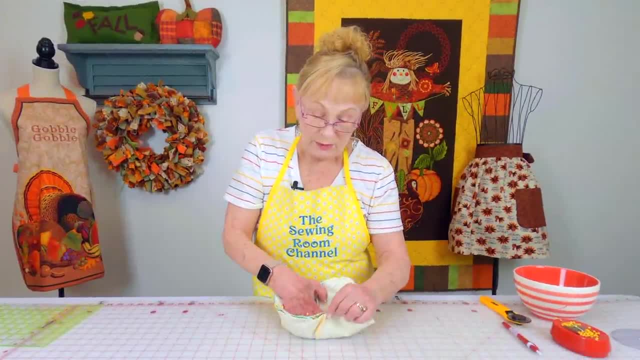 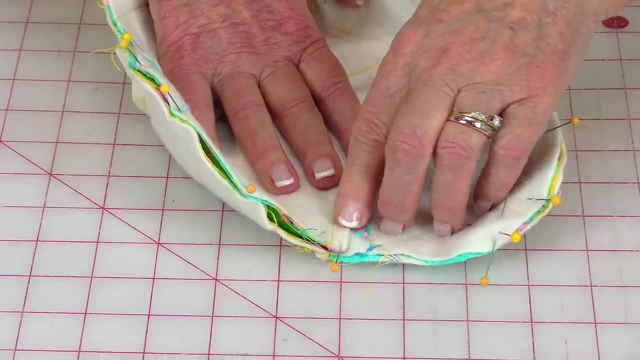 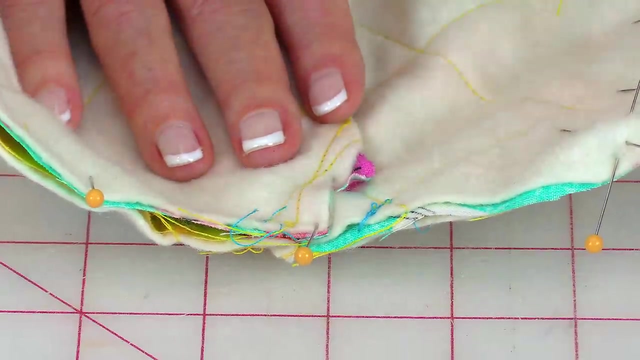 As you're pinning, when you come to your seams, you want to match the seams up Now to make it easier to stitch over these little seams right here, I pinned one seam going one way and the other seam going the other way, and that way it's not too lumpy. It's hard to open up these quarter inch seams, so that's why I did it that way. 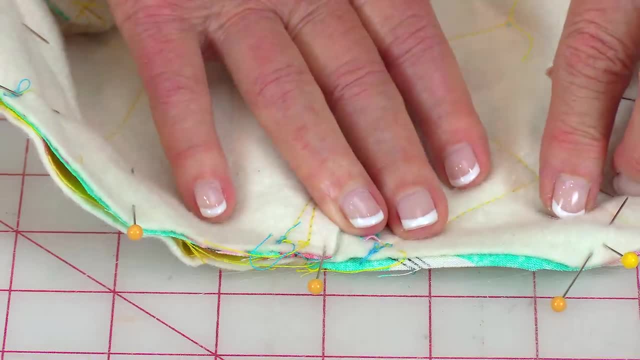 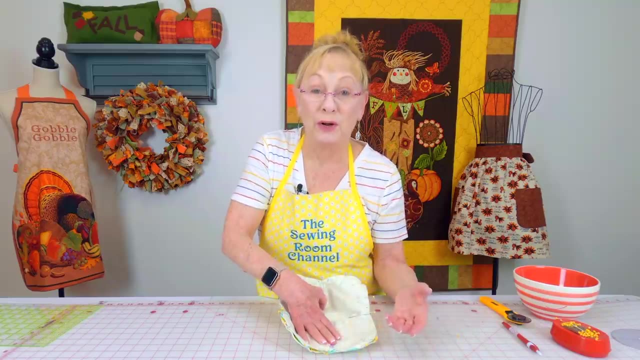 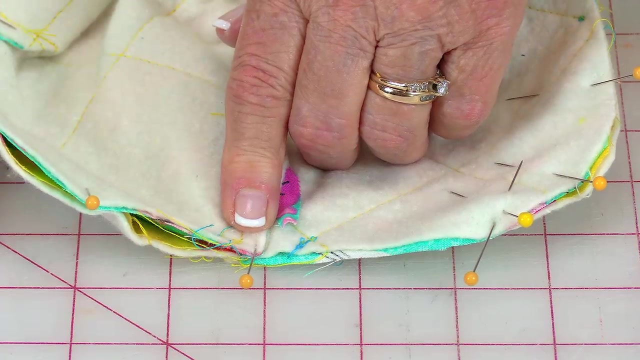 So place pins all around the edges, Then indicate one area- and this is my area. I have right here where you're going to leave it open. That's because we're going to turn it front side out, So I'm going to start here at this seam and stitch a quarter inch all the way around. 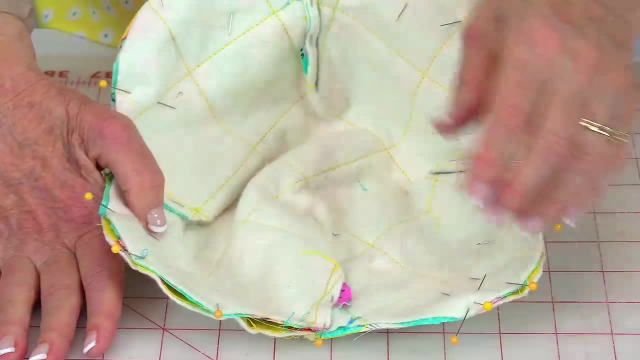 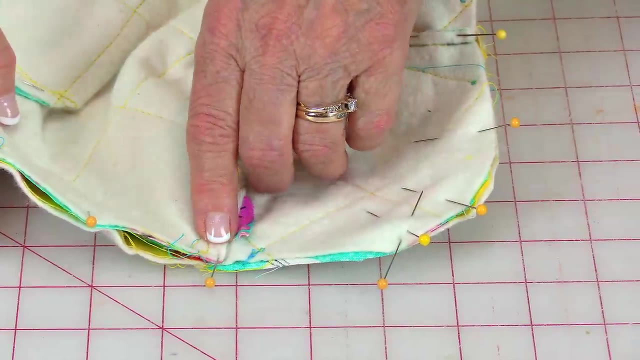 Now, when you get to the corners, you want to go a little slow, and I've got two pins over here and this is where I want to stop. So back, stitch at both the starting point and the ending point. After stitching, then you want to go around. 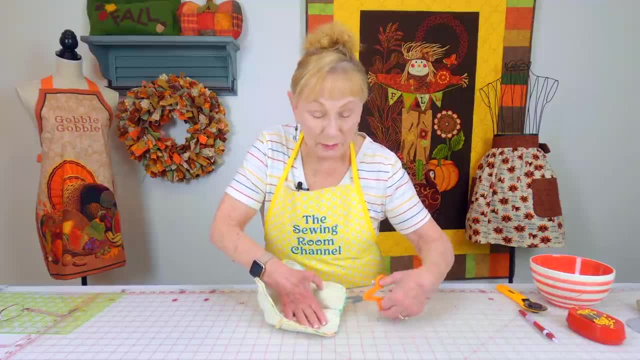 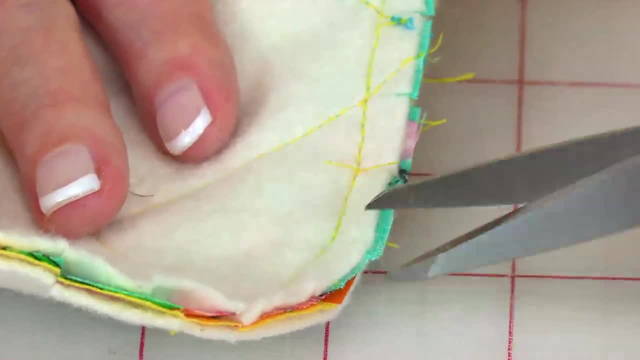 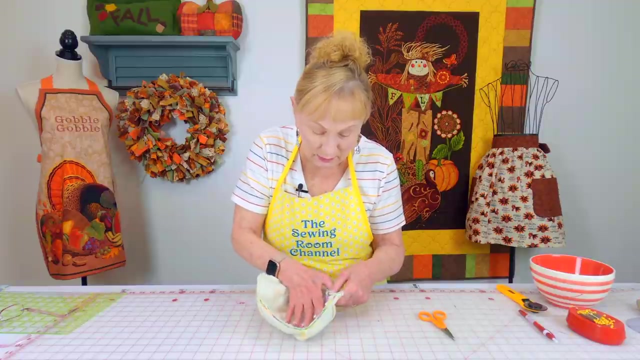 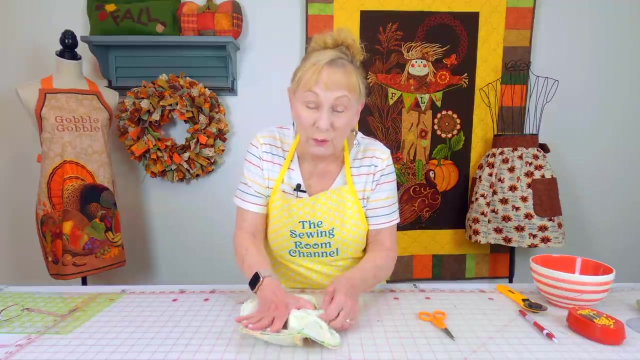 So I'm going to go around all of the edges- and with some small scissors it's much easier. Just do little clips, cut right up near- not through- your stitch line, and do these little clips all the way around the edges. Then you're going to go to wherever your opening is- Here's mine- And you're going to slowly begin turning it front side out, because all you've got is this little opening. so it's going to take you a little bit to do it. 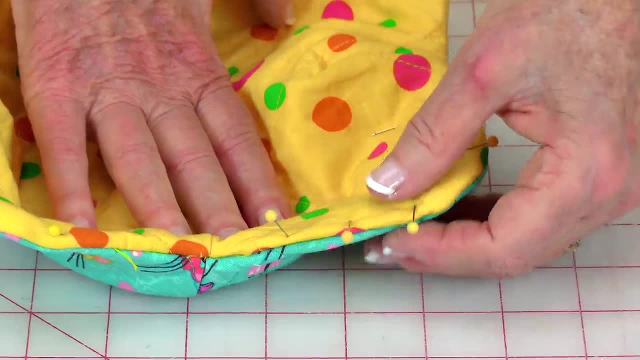 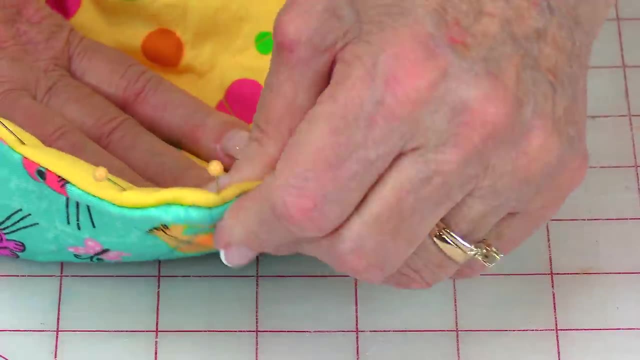 So here's where my opening was. So you want to turn those edges inside one quarter inch and pin it closed? Then I went ahead and pinned my edges flat because it's going to be a lot easier to sew them, because it's really thick. 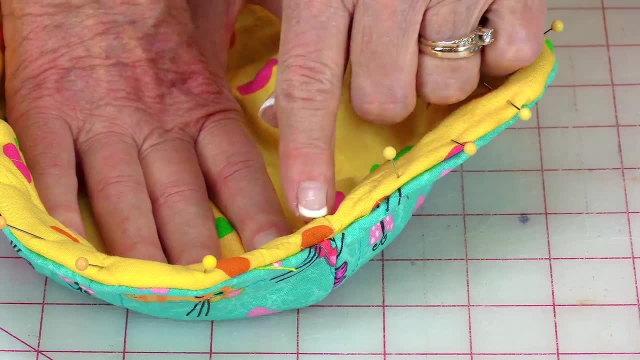 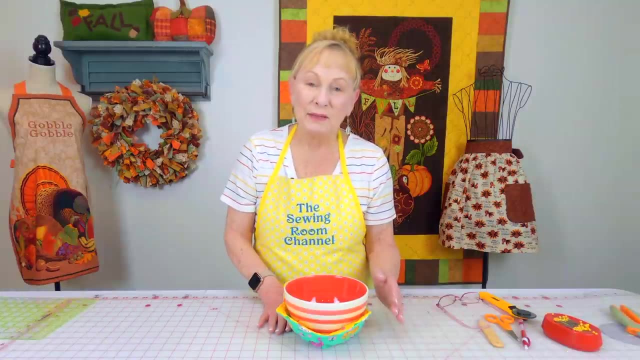 So you want to not only just stitch over your opening, but you want to go all the way around the edges, and you're going to do about a one eighth inch seam. As I was stitching around the edges, I had my stitch length set at three. 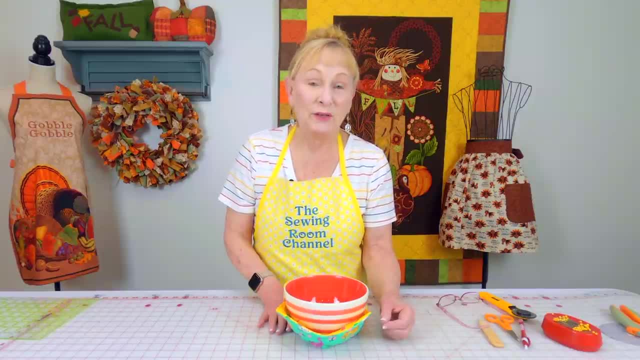 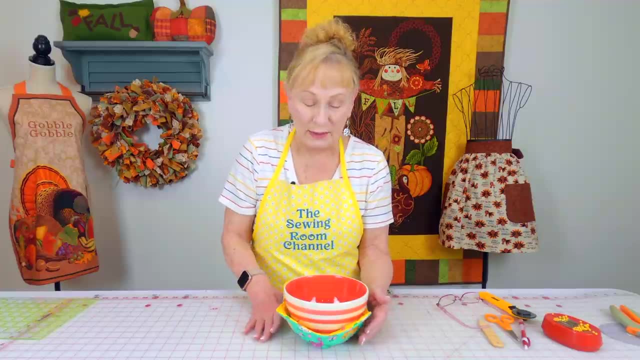 But it was so thick I had to adjust it And I changed it to 3.5.. So you may want to just stitch a little bit and see if it's working out for you, if you need to make adjustments. And this is how it turned out. 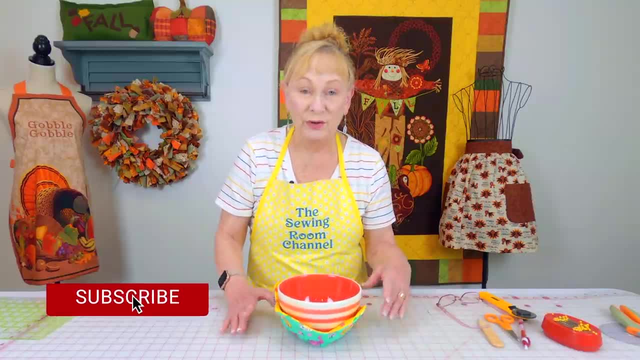 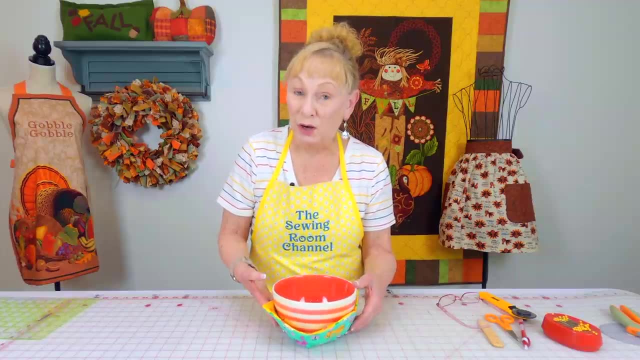 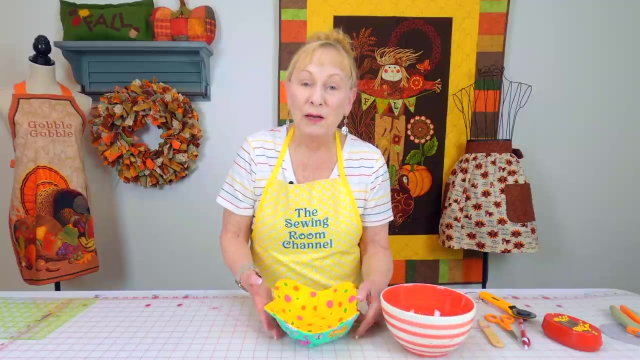 This is really, really cute. You can always make these larger or smaller. The best way to adjust the bottom is to just adjust your darts, Either shortening them or lengthening them just a little bit. One thing that's nice about this microwave button. 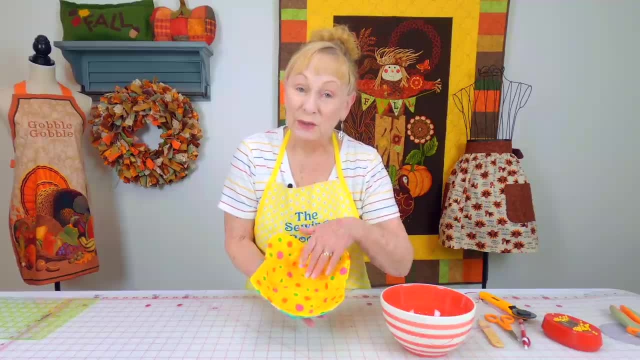 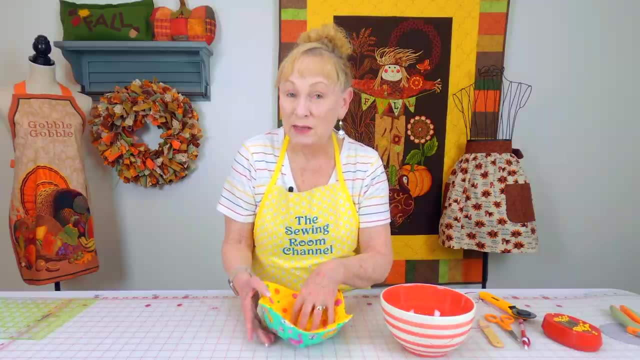 Bowl cover is that it's a different color on the inside so you could just turn it the other way, And on the outside I have little kitty cats, So you can make these for children. You can even put little snacks in here, like pretzels or little popcorn. 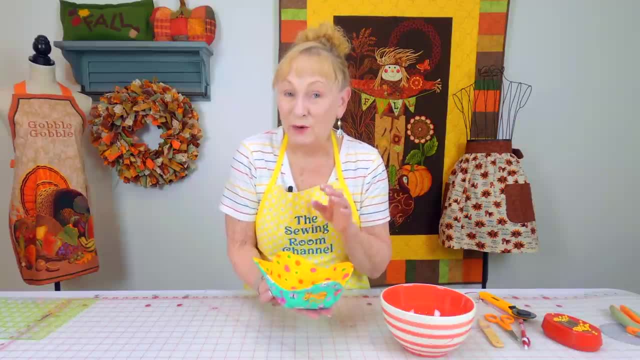 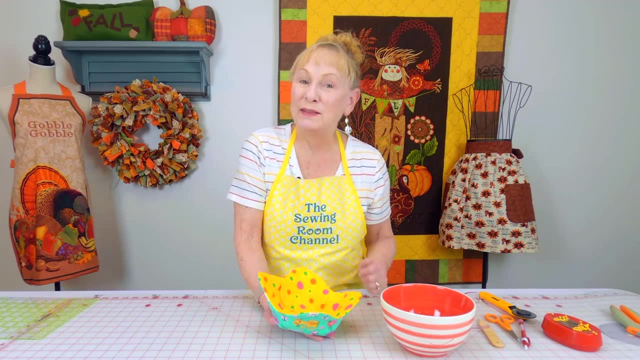 I have another friend who's a grandma, and that's what she does. Not only does she use them for her bowls, but she gives them to the kids with their little snacks in it. Now let's move on to the next project We're going to make the baked potato bag. 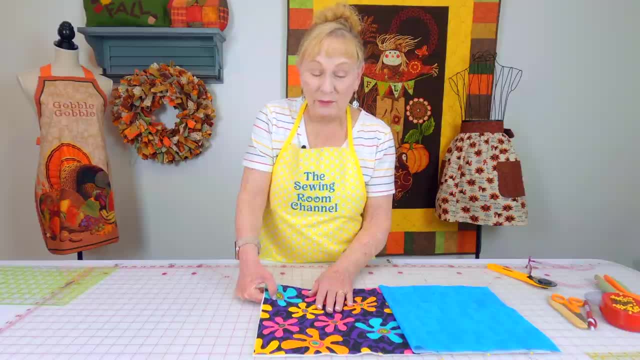 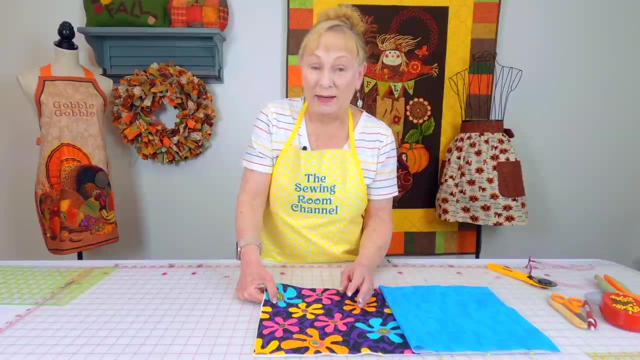 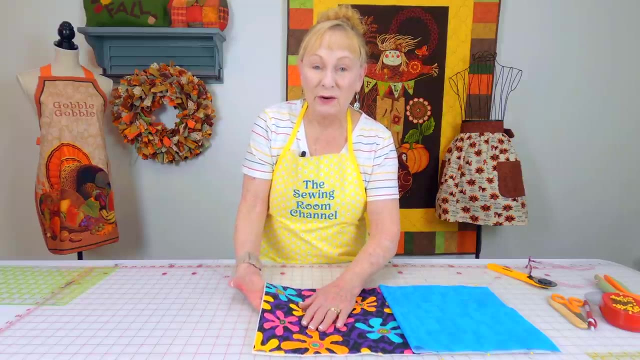 You'll need two rectangle pieces of fabric that are both 10 inches by 20 inches. You'll also need one cotton batting layer that is also 10 by 20.. So I've put the cotton batting underneath this layer here. This is going to be my outside. 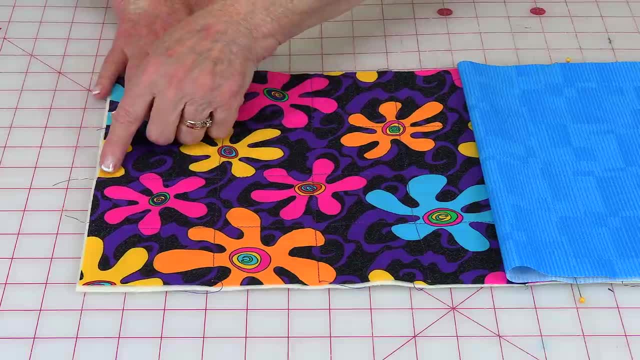 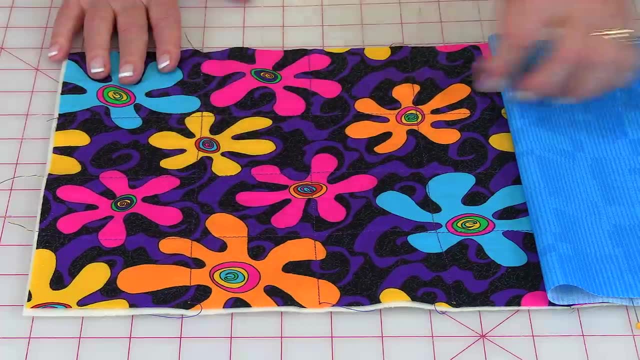 And I did some quilting stitches on it. I went in the middle here and went all the way down to the other end. Then I went over one more on each side and went down a couple inches apart, And then every few inches I did one like this: 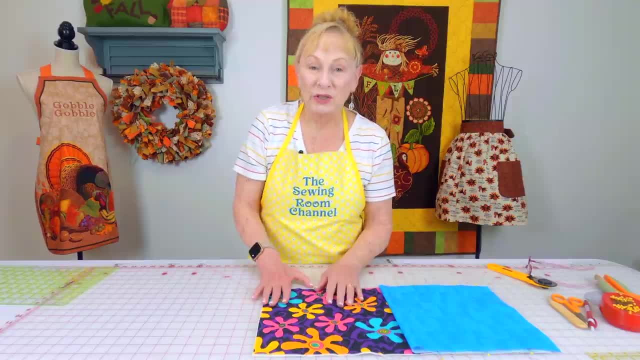 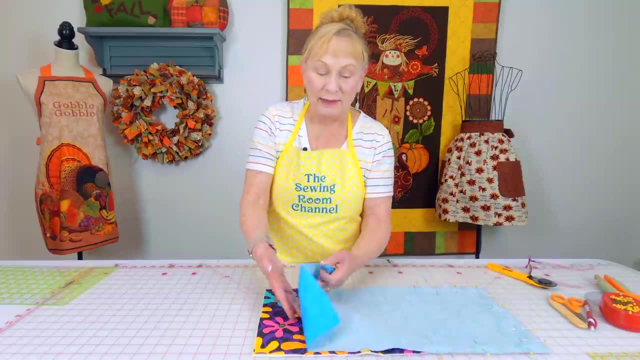 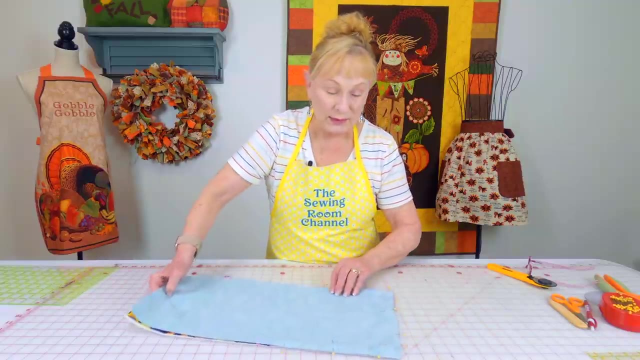 This helps to hold that cotton batting in place, so when you wash it the cotton batting doesn't shift around. So after you've got that done, then take your other piece of fabric and lay it on top, And then you're going to place pins all the way around, all four sides. 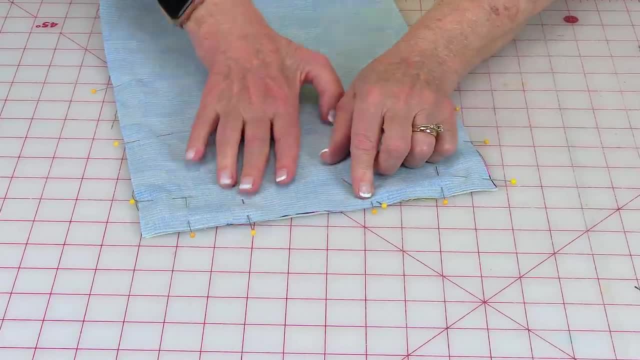 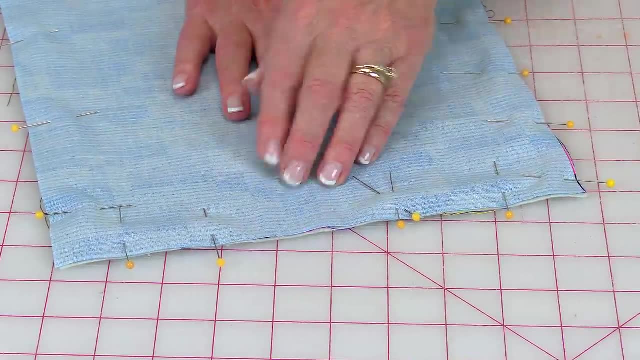 And always indicate where you're going to leave it, Leave an opening. So I have two pins here and one pin here, And this is where I'm going to turn it, front side out, And this is my starting point. I'm going to back stitch here and also back stitch at the end. 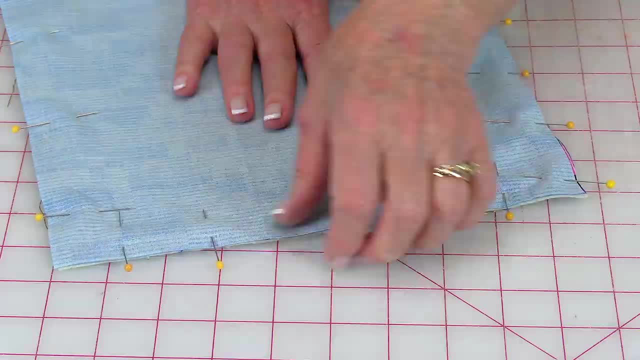 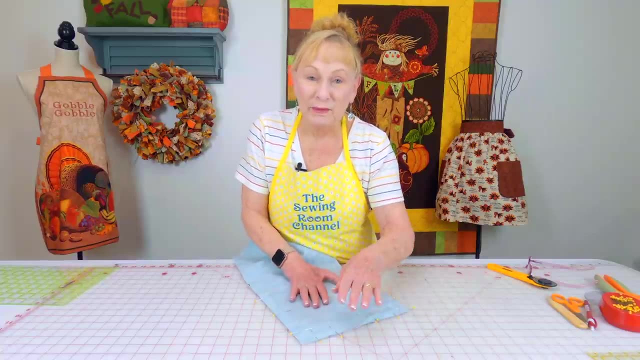 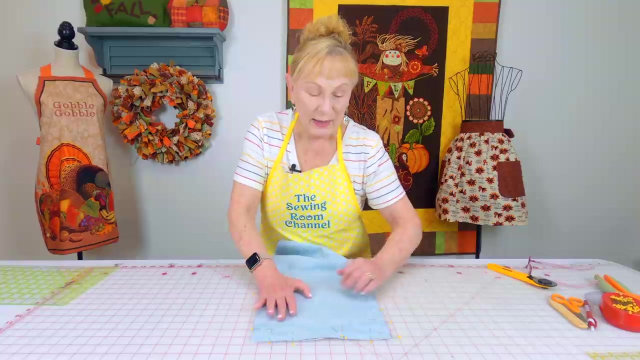 You'll do a 1 quarter inch seam starting here. As you go down to this corner right here, leave your needle down through your fabric, Lift your presser foot, Turn this fabric here, Lower your presser foot and continue stitching. Cut at all your corners. 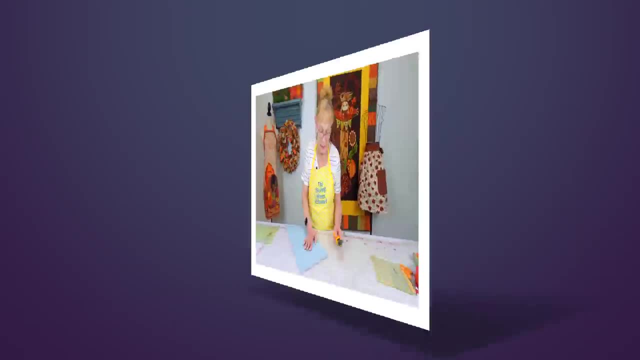 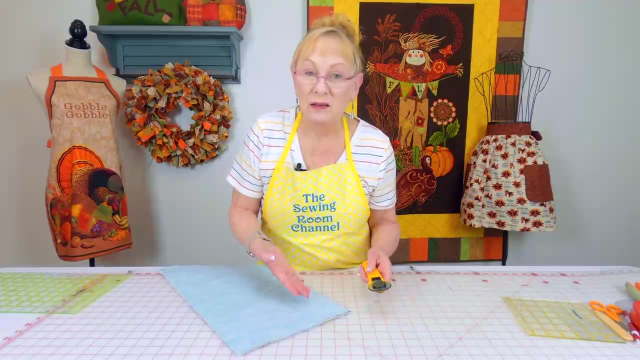 And when you come back around here, don't forget to back stitch. Now you want to trim some of the fabric off the corners, Because if you don't do this, they're going to be very thick and lumpy And they're not going to lay very nice. 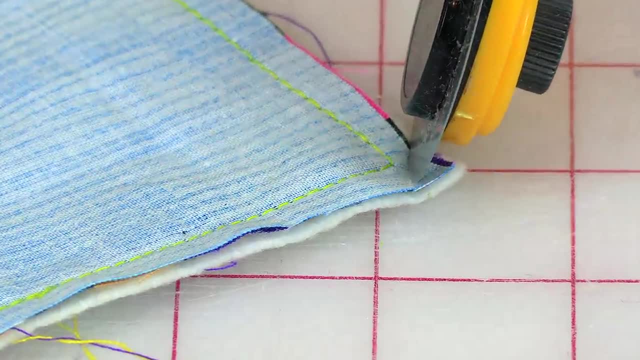 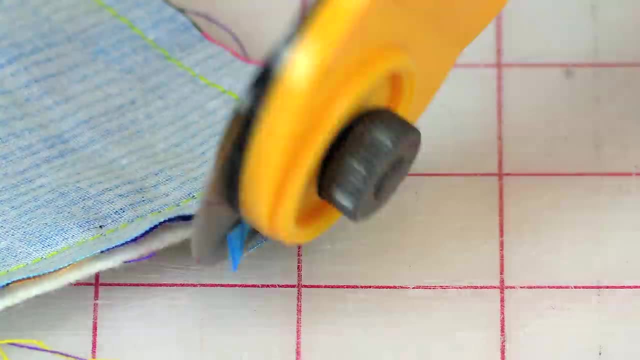 So I like to cut them down to where they're about an eighth of an inch wide. So I'll cut some going off this way And then I'll go off to the side and just trim a little bit of it off, And also on the other side. 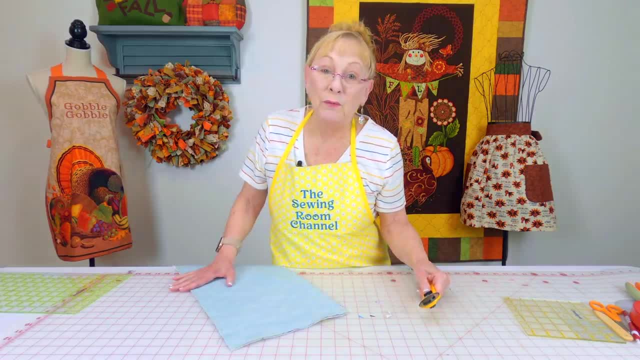 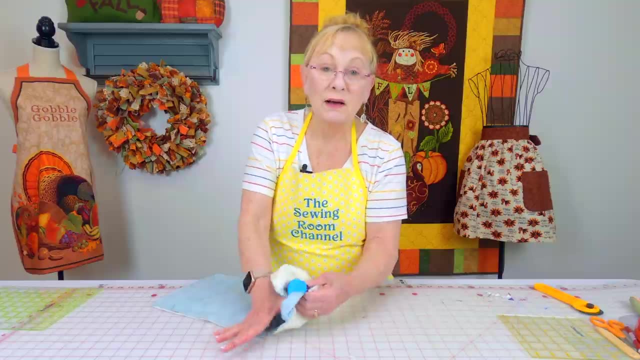 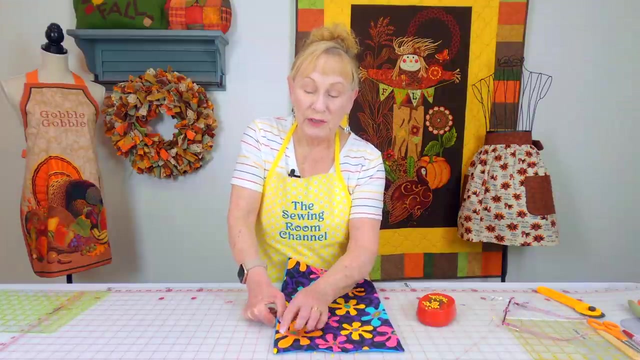 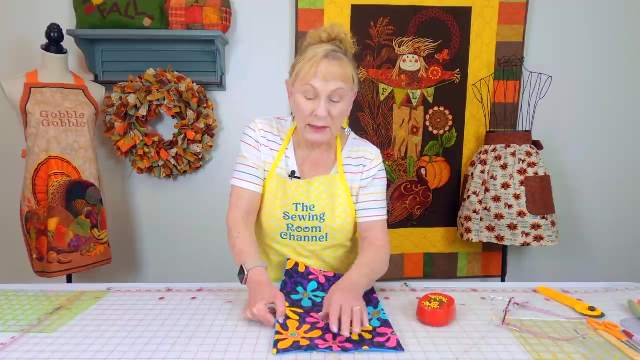 I'll do the same thing And again, do this at all four corners. Now go through your opening and begin pushing the front side out. Before you close up your opening, you want to reach inside and poke all four corners out To make sure that they're flat and not too rounded. 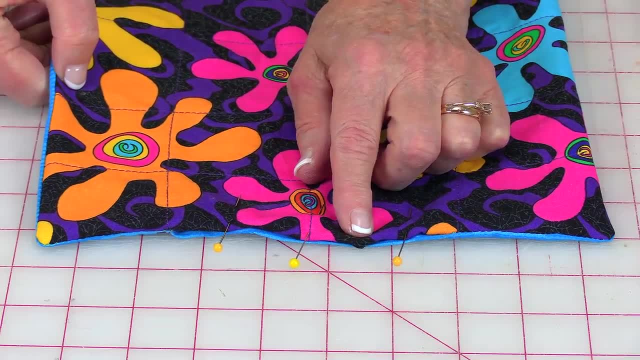 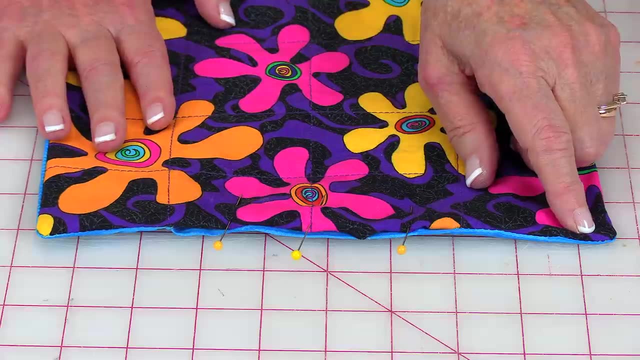 Then pin your opening closed by turning the edges in 1 quarter inch And you're going to go around and not only are you going to stitch across here, But you're going to stitch close to the edge all the way around, all four sides. 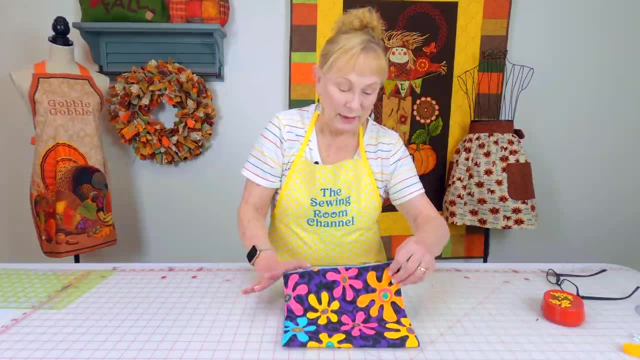 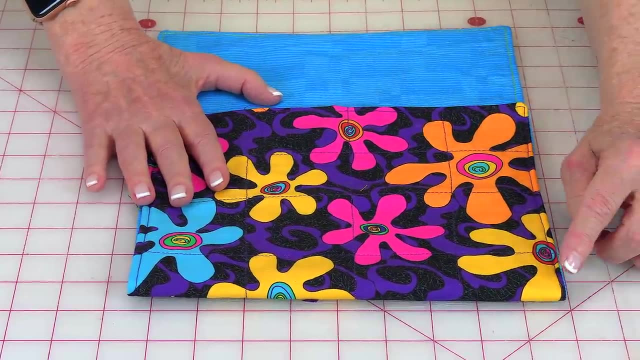 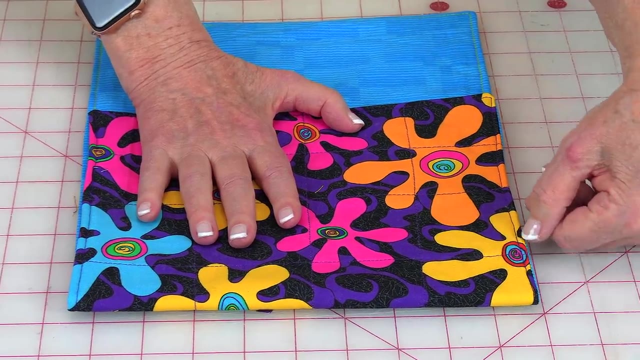 Now you want to fold it up And I went up about 7 inches. You could go up 8 if you wanted to. So there's about 7 inches from the bottom up to here, And this last step is really easy. You're just going to stitch right over the same stitch line.